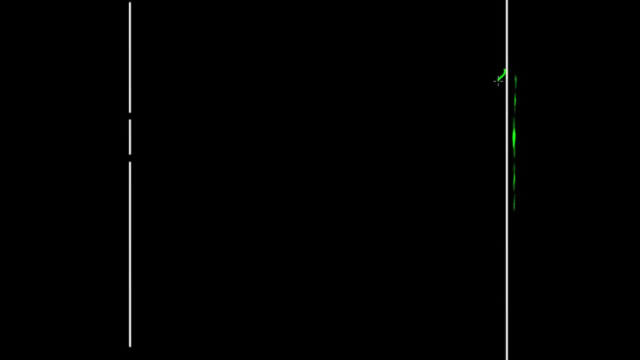 which is why, when we draw a graphical representation of this, it kind of looks like this, where these spots are blending into each other, which is cool, but it also kind of sucks, because if you were to go actually try to do this experiment, you'd want to measure some angles. 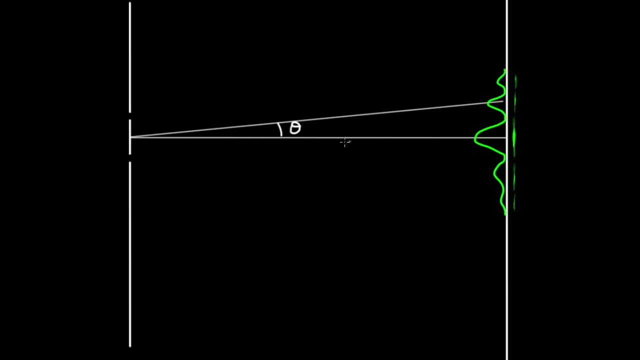 And that means you have to measure some distances. I'd measure distance from the screen to the wall. That would give me this side of the triangle, And then I'd also probably want to measure distance between two of these bright spots, because that's what I can see, but because they're smudgy, it's like. 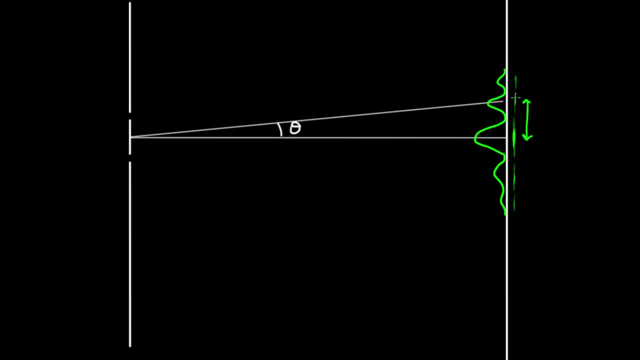 is that the center? Is this the center? Sometimes the light's not so strong and it's hard to tell, And what's worse is these kind of die off, And so this is another problem. These die off pretty quick. Sometimes you're lucky to even see the fifth or sixth bright spot down the line. 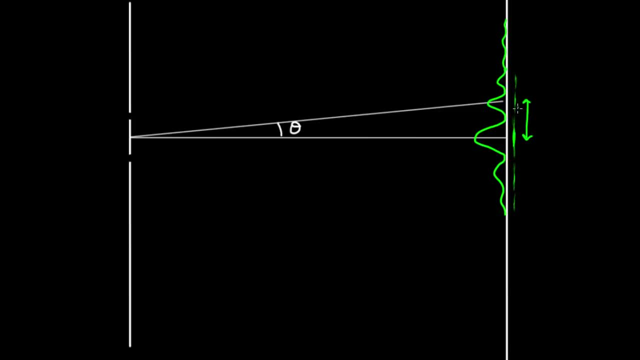 So my question is: is there a better way? Is there a way to make these spots more defined so you can see more of them, so they're brighter? And the answer is definitively yes, and we figured out how to do it. The way you do it is, you just make more holes. 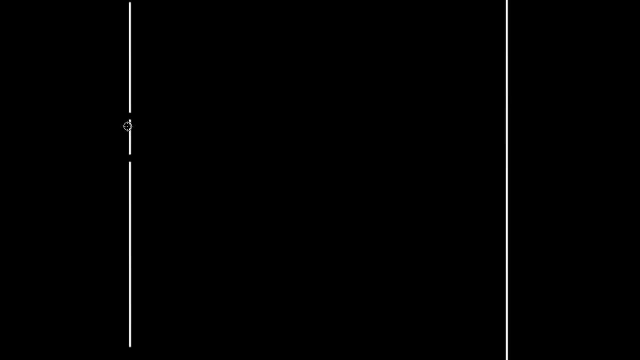 So you come over to here and if these are spaced a distance d, I'm just going to make another hole a distance d, And then I'm going to make another hole a distance d, And then I'm going to make another hole a distance d. 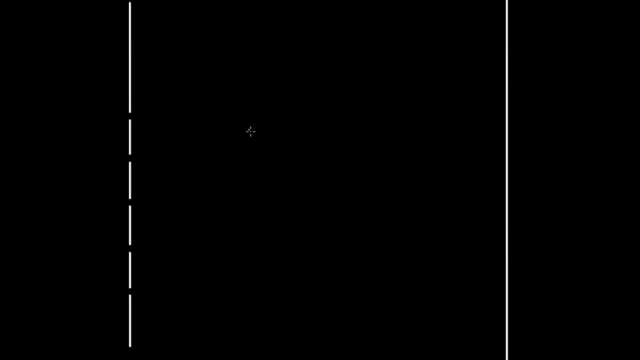 I'm going to make hundreds, thousands of these holes extremely close together. As long as they're all a distance d apart, something magical happens. So if these are all d apart, what happens is on the wall over here, instead of getting this smudgy pattern. 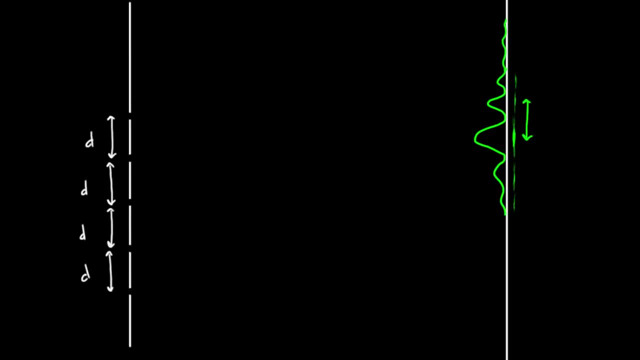 you'll get. you really will just get a dot right at there, and then darkness, and then another dot, and then darkness and another dot, and you'll see this continue out much further than you could previously. Why? Well, let's talk about why. 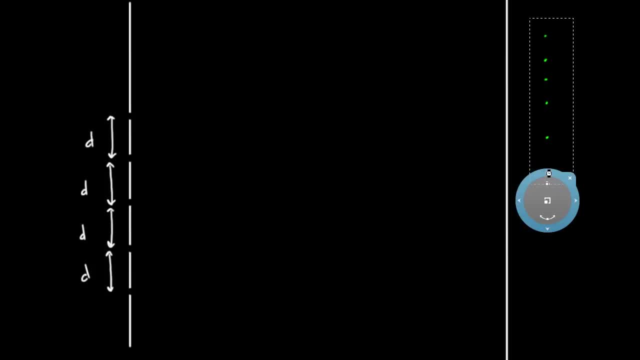 So let's talk about this. How come you see this pattern over here like this? So the first wave from this first hole- let's imagine this first wave from this first hole- it's going to travel a certain distance to the wall. Let's say we look at a point over here where it is constructive. 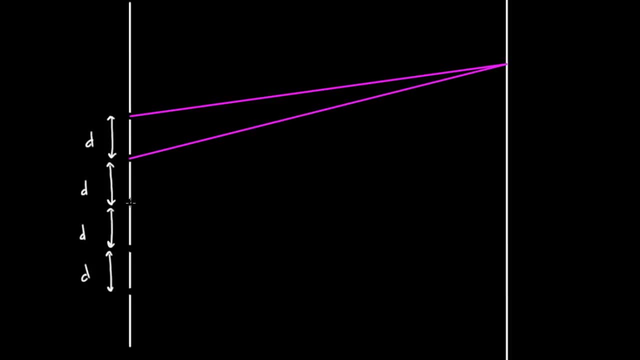 Let's say we just have these two holes to start off with right, Two holes double slit. disregard all this stuff for a minute. Two waves coming in from two holes, get over to here. Let's say this is a bright spot. 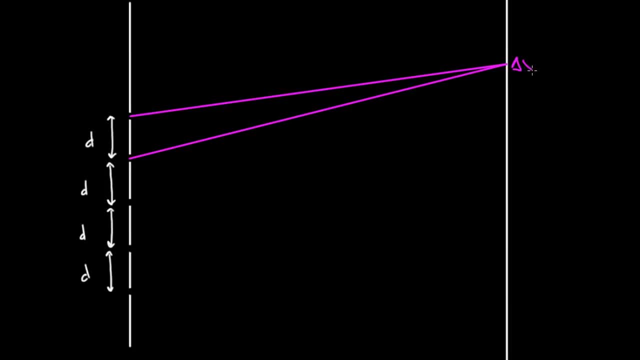 Let's say it's the bright spot that corresponds to delta x equals one wavelength. In other words, this would be the constructive point where the second wave from the second hole travels one wavelength further than the wave from the first hole. And again, what that means is if I were to carefully draw a line from here at a right angle, right there. 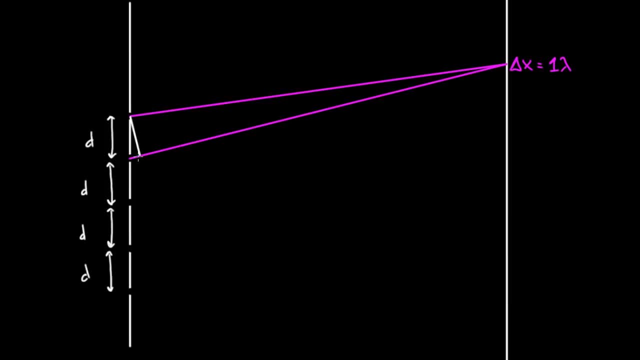 that means that this wave from the second hole, this is the extra part, So that would be one extra wavelength. And because this second wave is traveling one extra wavelength, it's going to be constructive because if I draw my wave they're going to match up perfectly there. 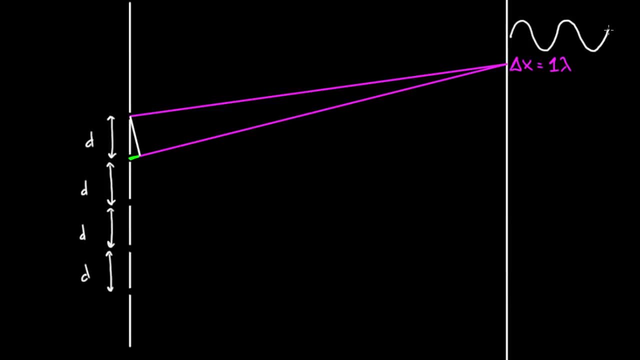 So if I draw my wave, let's say the wave from the first hole happened to be at this particular point on its cycle. It doesn't have to be, but let's just say it was there. The first wave hit that point at this point in its cycle. 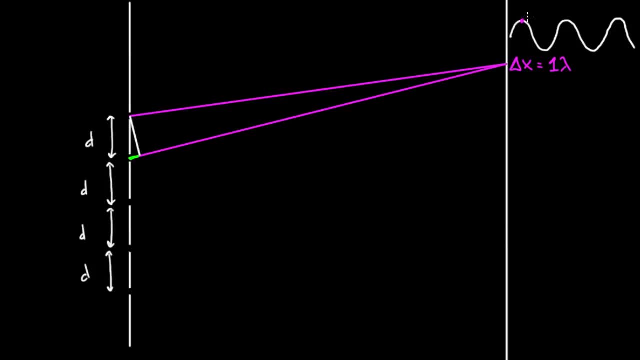 Well, the second wave, since it's traveling one wavelength further, is going to hit at this point in its cycle, So it would be here Now. these are both hitting there at the same point, So the first wave gets there hitting right here. 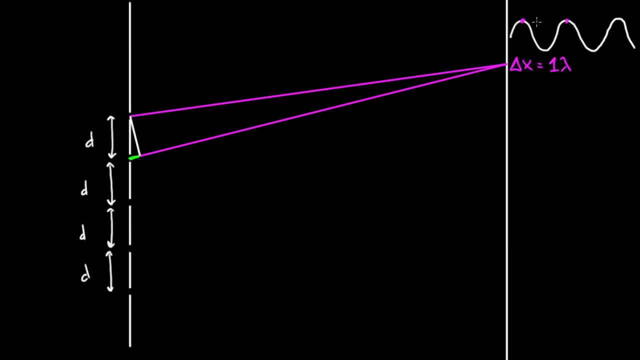 The second wave gets there hitting right here. These overlap Because these are two different waves overlapping at this point It's going to be constructive, because if a peak matches a peak, constructive, If a valley matches a valley, constructive. How about the third hole? 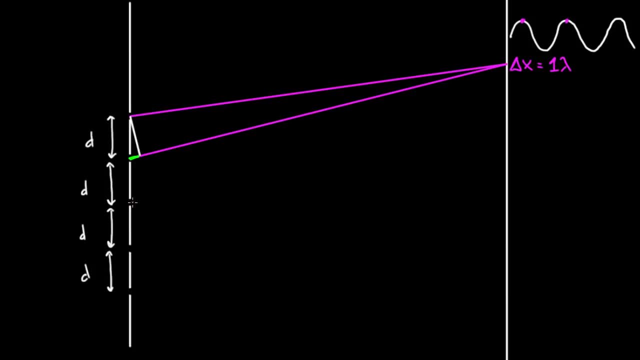 Here's where it gets interesting. This third hole, the wave from the third hole, is going to have to travel this far to get there. Well, let's see From the second. how much further does it travel compared to the second hole? 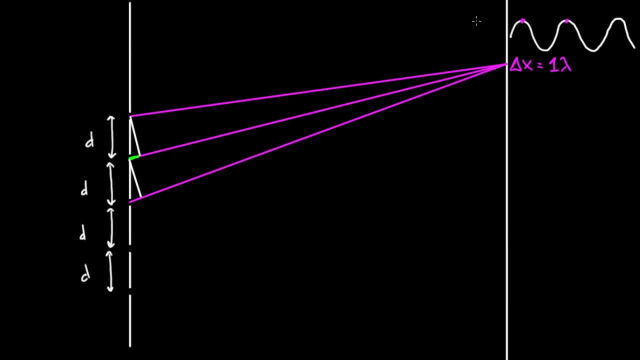 I'm going to do the same game I did just a minute ago. It travels this much further, which, again, since these are the same angle, this is going to be the same distance here. This is also going to be one wavelength. Remember we derived this that d sine theta is the path length difference. 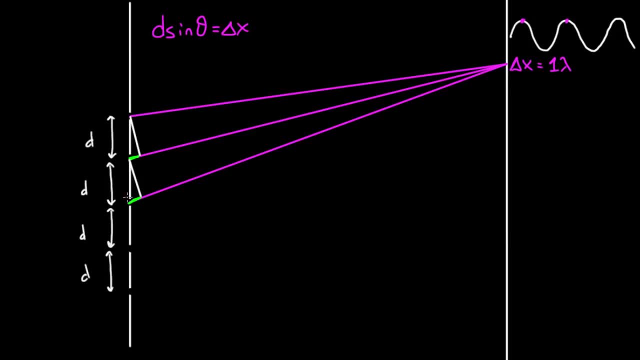 And the theta is the same for all of them, And so I could just look at these two, consider these two as a double slit. This one travels one wavelength further than the second. How much further does it travel than the first? Well, I'm going to continue that line down. 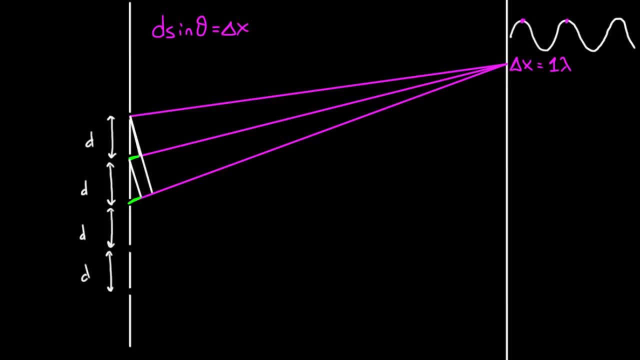 It's just going to travel two wavelengths farther than the first. So the wave coming out of the third hole travels two wavelengths farther than the first hole. The second and the third are going to be constructive because they're one wavelength apart, And the third and the first are going to be constructive because they're two wavelengths apart. 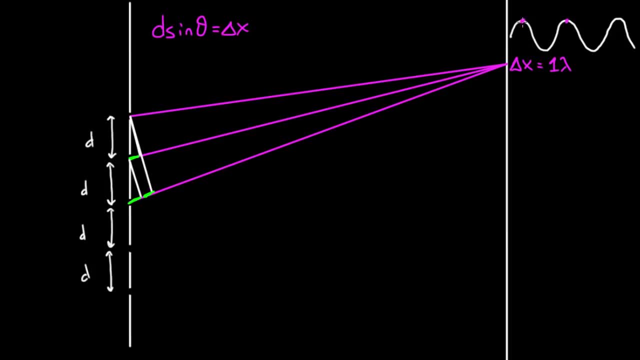 That's okay. Two wavelengths, it doesn't matter. Look it, If the first one hits here, the wave from the second hole hits here, The wave from the third hole travels two extra wavelengths. When that third wave gets to this point, it'll be at this point on its cycle. 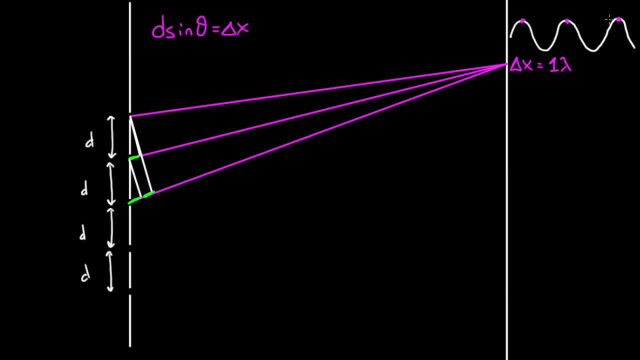 They're all going to be overlapping at the same point on their cycle. It's going to be constructive. You can keep doing this, You can come down to this hole and it'll also be constructive interference. In other words, this fourth hole travels one wavelength further than the third. 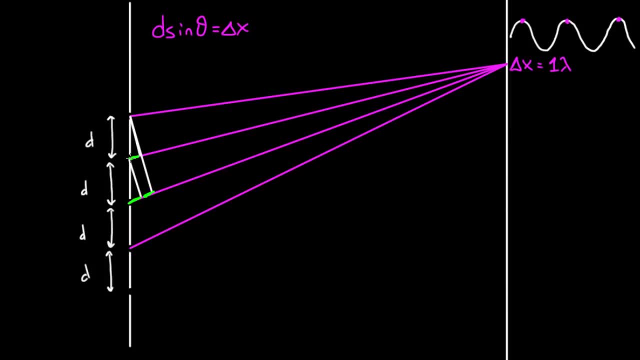 Two wavelengths further than the second hole, Three wavelengths further than the first hole, But they're still all going to overlap perfectly. You will get an extremely bright spot here, Because now you have even more light overlapping And it's all perfectly constructive. 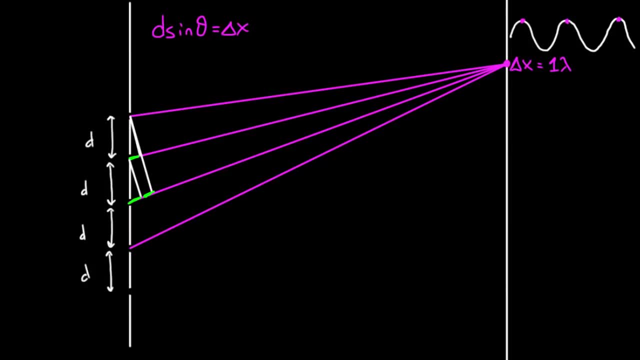 Bright spot. Now here's where it gets strange, So you've got to be careful. This is the part of the explanation I hated as a student. I thought this made no sense whatsoever, So pay close attention at this point. Here's the weird thing. 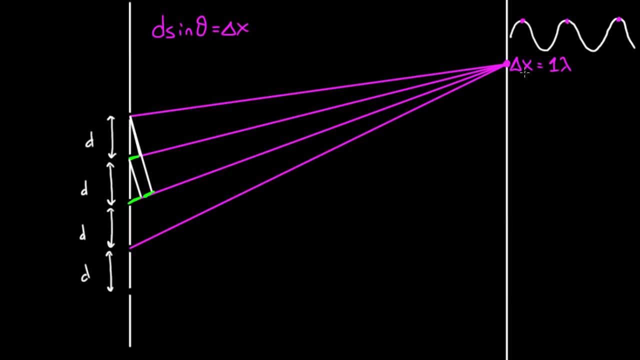 If you deviate slightly from this constructive point, If I go up just a little bit over here to some point right here, Let's just see what happens. This wave from this first hole would travel that far to get there, Okay, And the wave from the second hole travels that far to get there. 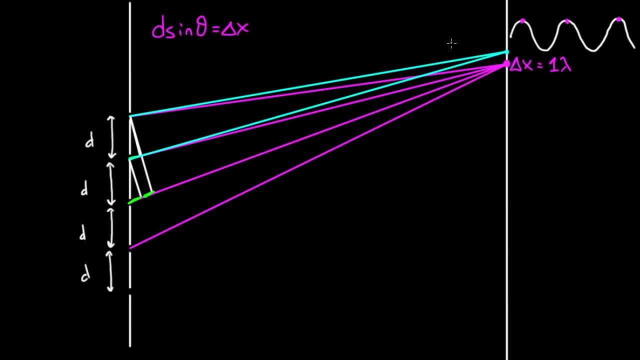 The path length difference isn't going to be one wavelength. Let's say the path length difference happens to be 1.1 wavelengths. So let's say the wave from the second hole happened to be traveling not one wavelength further anymore. It's not traveling one wavelength further. 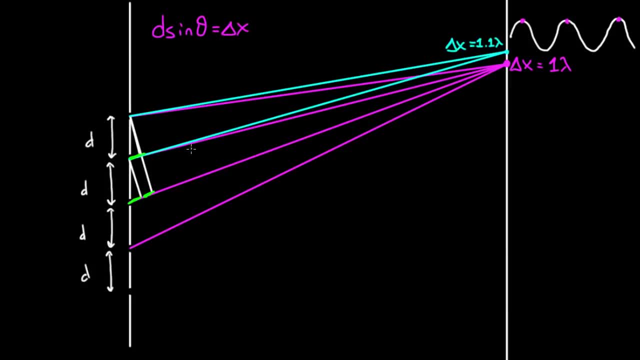 It's going to be traveling one and 0.1 wavelengths further, And so if the first wave happened to hit at this point, The second wave would be hitting at not exactly one wavelength, But 1.1.. Now, if I keep drawing them over here, I'm going to run out of room. 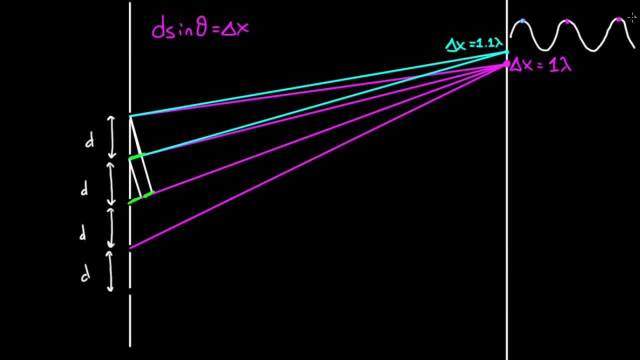 So since they're all the same points on the cycle, The cycle is the same over and over One wavelength: 0.1.. I'm just going to draw that right here, So the second wave would hit right there. Those would overlap. 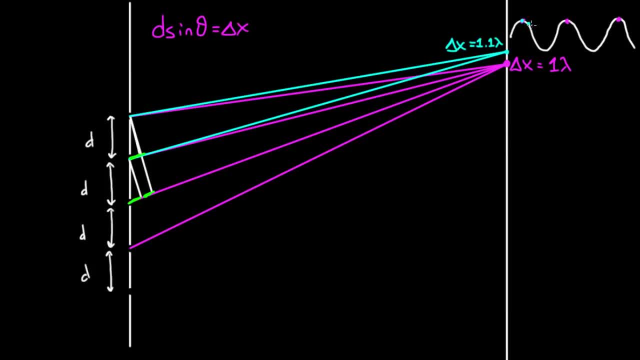 You know that's partially constructive. I mean you're going to get a. Just looking at these, you'd think you'd get a bright spot, But if you keep going, Let's see what happens. Wave from the third hole also travels to get there. 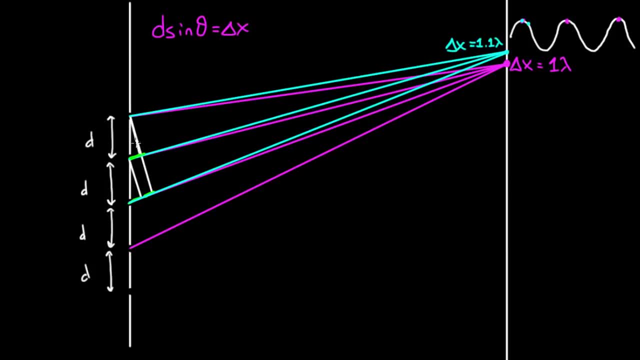 How much farther does it travel? Well, it travels 1.1 wavelengths further than the second hole, But it travels 1.1 plus 1.1 wavelengths further Than the first hole, So it travels 2.2 wavelengths further than the first hole. 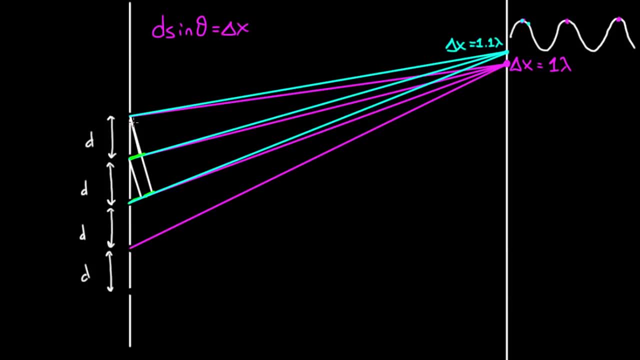 So to make this clear, Let me just be clear here. So if I do the same trick Right, I draw this down to a right angle. It's a little farther, So I have to draw the line a little further out. First wave travels: 1 wavelength. 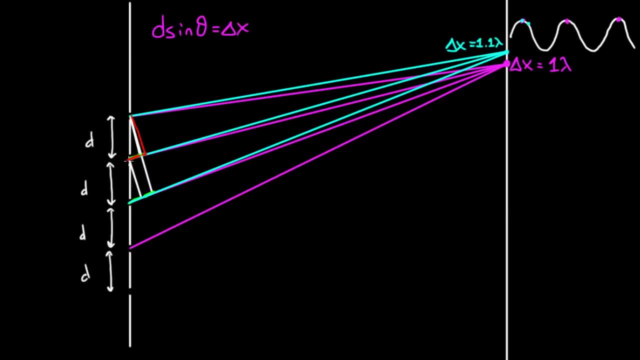 And 0.1 wavelengths further. How about this one here? Well, The wave from the third hole travels 1 wavelength, 0.1.. 1.1 wavelengths further than the wave from the second hole, But it's going to travel. 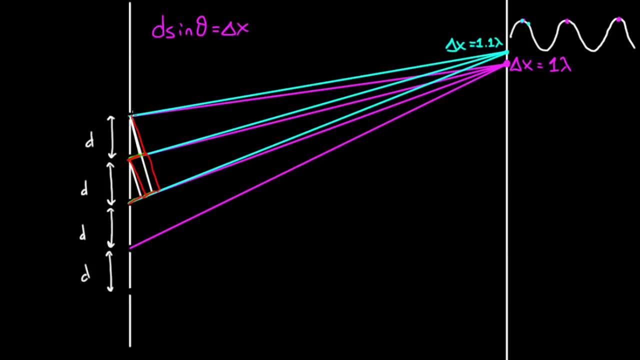 1.1 plus 1.1 wavelengths further Than the first hole, So it's going to be 2.2.. This wave from the third hole Is going to travel 2.2 wavelengths further Than the wave from the first hole. 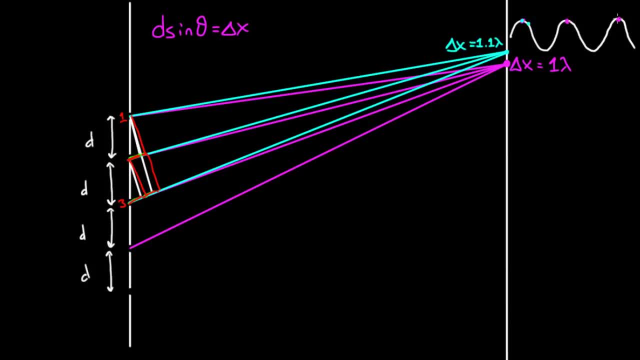 Where would that be? So 1., 2 wavelengths, 0.2 would be even further down the line here, Not completely to the bottom, But further down the line. So it would be At this point over here And you can keep doing this. 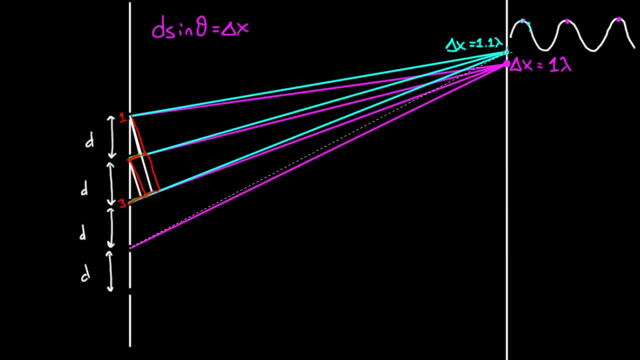 And let's just see what happens. Let's just do a couple more. This wavelength has to travel this far. So now you can probably see the pattern. This wave through the fourth hole Has to travel 1.1 wavelengths further. 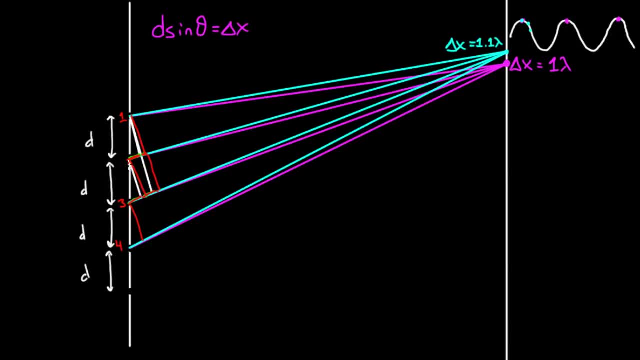 Than the wave from the third. It travels 2.2 wavelengths further Than the wave from the second, Travels 3.3 wavelengths further Than the wave from the first. So if I compare this wavelength Where this wave is on its cycle. 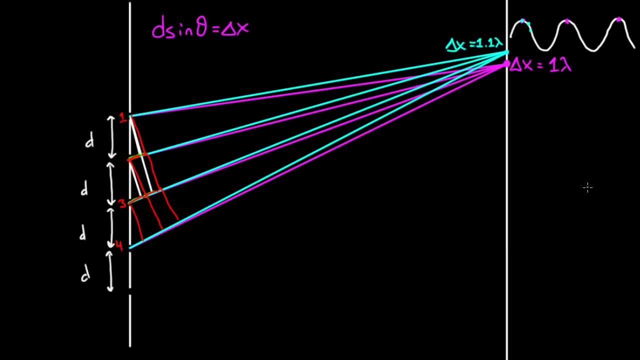 Compared to the first, Then I'm going to be 3.3 wavelengths. So if I go 1,, 2,, 3. And then 0.3.. It would be down here somewhere I'd get one that's at 0.4.. 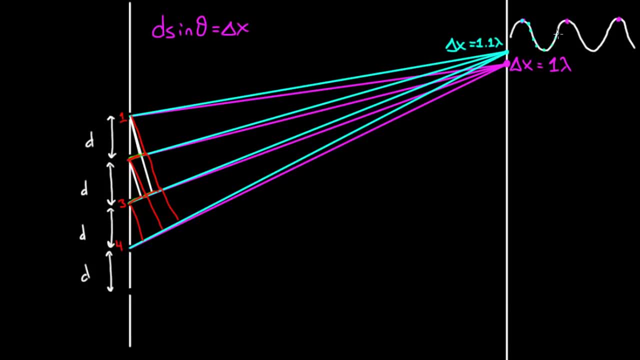 I'd get one that's at 0.5.. I'd get one that's at 0.6.. One at 0.7.. One at 0.8.. One at 0.9.. One at Well, 0.10.. 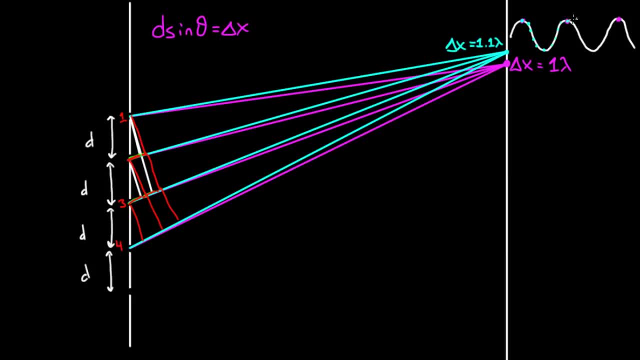 Back to A whole wavelength Wavelength, again, A whole wavelength difference. What is this going to be If all these waves are overlapping like this At this point? That's only slightly deviated From this other point. What am I going to see there? 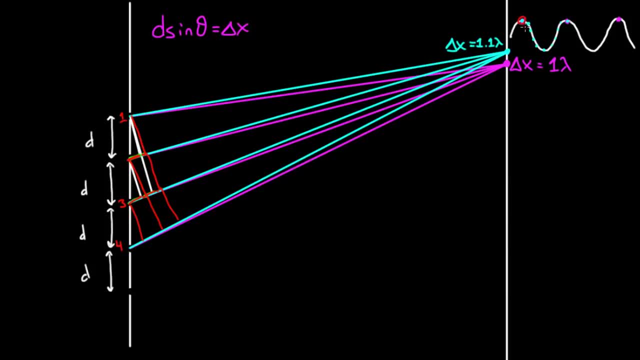 Well, This Look at You could pair these off. This point And this point Are going to interfere completely destructively. One's at a maximum, One's at a minimum, One's at the peak, One's at the trough. 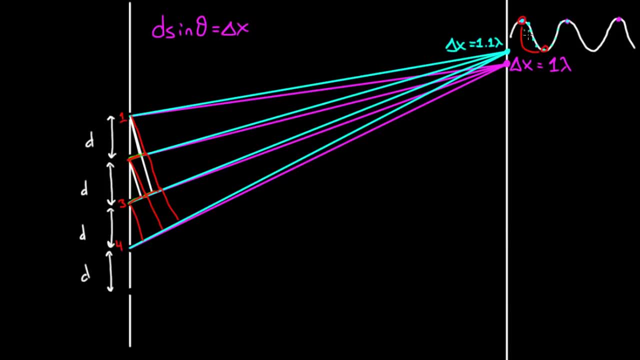 And so you get 0. And you can keep pairing these off, This one here And that one there, Completely, Completely annihilate each other, Completely destructive, And you can keep doing this, This one here And this one there. 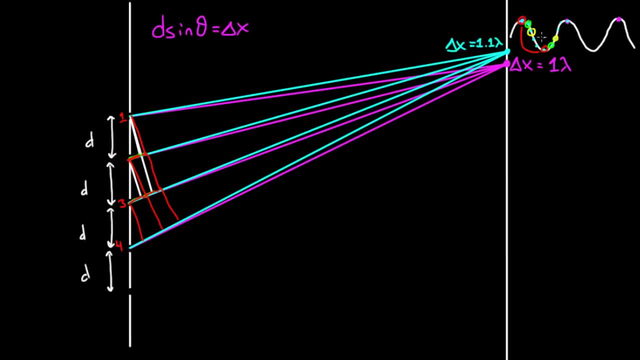 Completely destructive. You can keep finding points That completely destruct each other And that means You're going to get no Intensity at all, Even slightly Off From this magical point, This magical Integer Wavelength point. What that means. 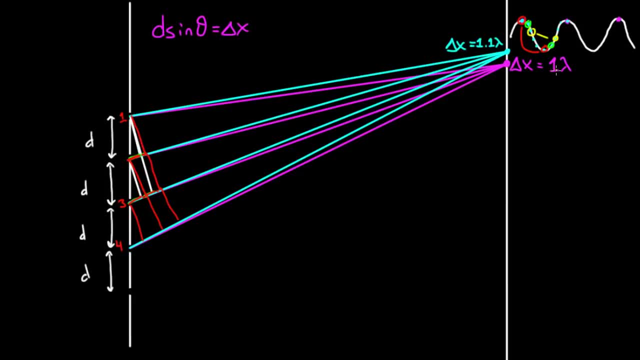 Is, instead of getting a blur, You're going to get A little bit of Distance From this Magical Point, This magical Integer. Instead of getting this, Instead of getting this Smudgy pattern, You're going to get 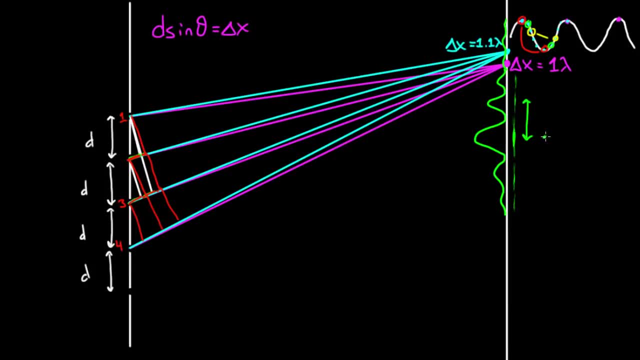 At the bright spots: A dot And then another dot At the bright spot, And in between These bright spots You will get Darkness, Which is great. It's great Because it's easier to measure, So that's one good thing. 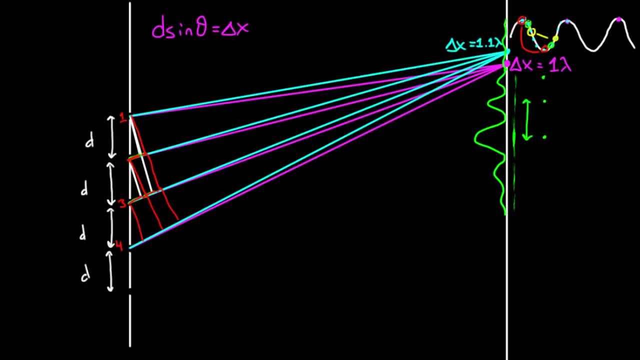 And it relies on this fact That if you've got Multiple holes, Hundreds, Thousands of holes, If you go off Even slightly- Because this Isn't going to always Match up points, You're going to get Distance. 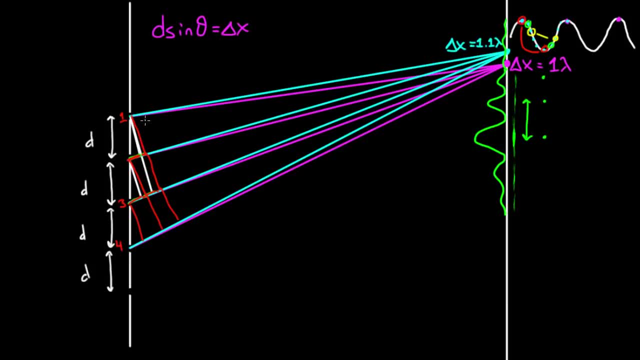 From this magical point To always Match up Perfectly. You keep going Down the line. One of these Are going to interfere Constructively With another, And you can keep Pairing these off. And then the second. 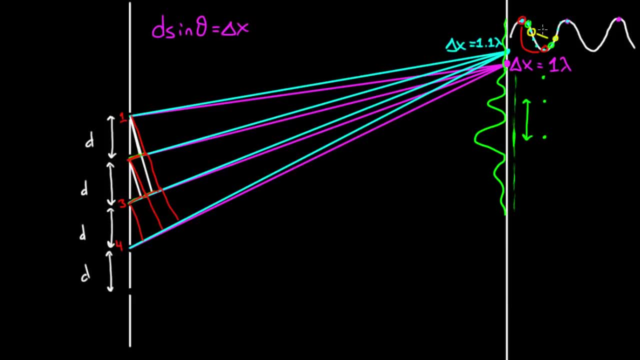 Would interfere Constructively With a different one, And the third With a different one, And the fourth With a different one, And they're always Going to match up So that you can Destroy them all And you get. 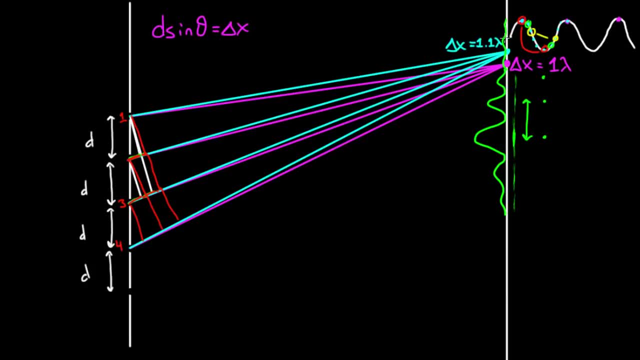 Destructive points In between. That's why it's dark Now. at first I didn't like that argument. I Try it out, Draw it out. I I've tried my best To explain it here, But I. 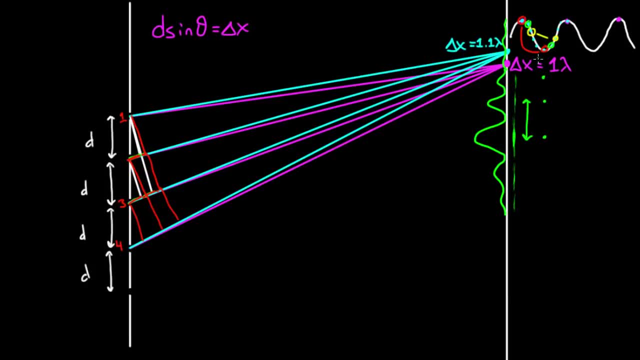 Have to admit It's a difficult one To sort of comprehend, But that's, That's the idea, And so This is great, Actually, These multiple Holes here Giving us points That are, Points that are. 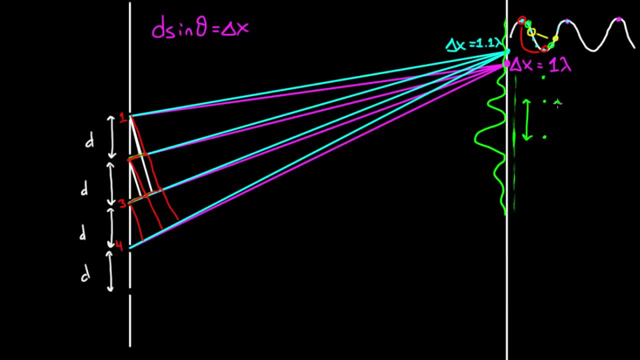 Spaced out And Clearly Delineated. Now I can clearly See. Okay, If I wanted to measure This distance, I don't have to guess. There's no guess work. One great thing About this. The other great thing. 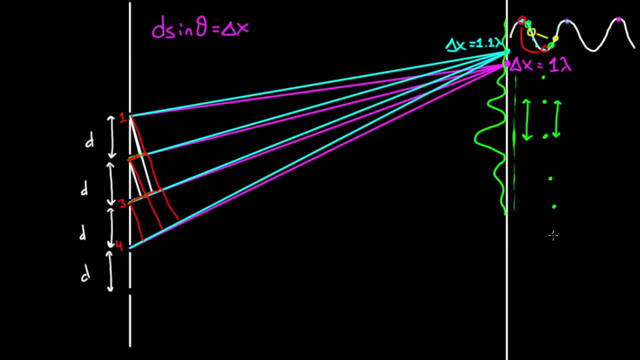 Is Because I've got more holes. This Brightness Lasts longer. These bright spots Will keep going Further. I can see this Travel further Down the line Than I would With this smudginess. 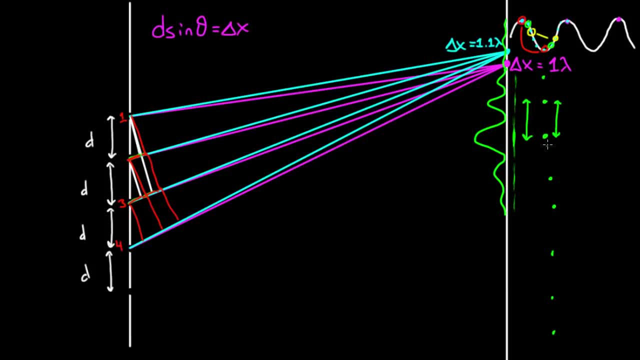 Because I've got multiple holes Interacting, I'll have more intense dots. It's brighter, So the dots Are more delineated And they're typically Brighter, More intense, And so We give this a special name. 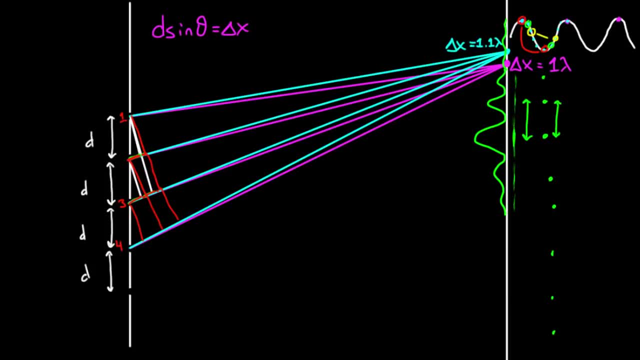 Because this is so useful, These multiple holes Are useful. We call this A diffraction Grading. So this is A diffraction Grading And it's More useful Than a double slit In many ways. 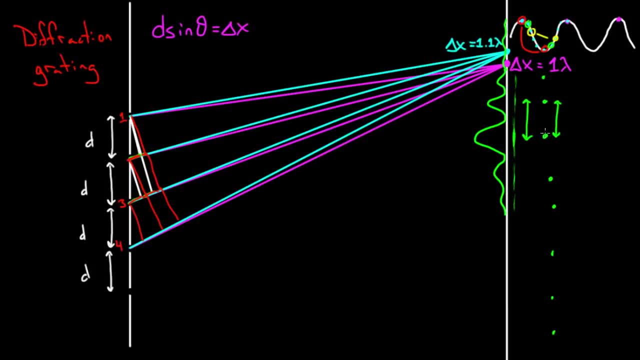 Because it gives you Clearly delineated dots And it lets you See them more clearly. And how many holes Are there In a diffraction Grading? Well, typically These are measured. These are rated In lines Per centimeter. 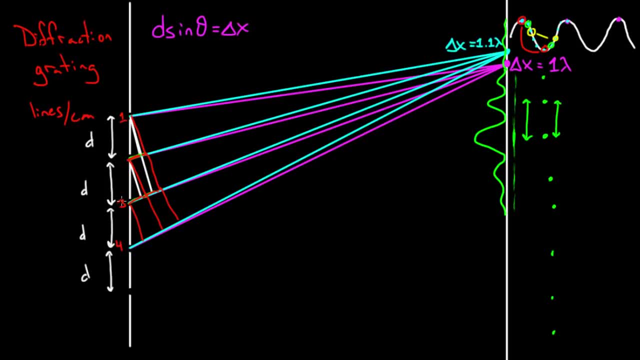 In other words, If you took A diffraction Grading, You asked: How many Holes are there Per centimeter? Well, The lines Could be The blocked parts And the holes Could be the parts.